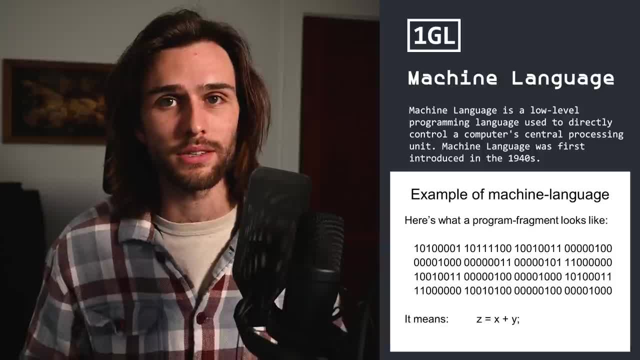 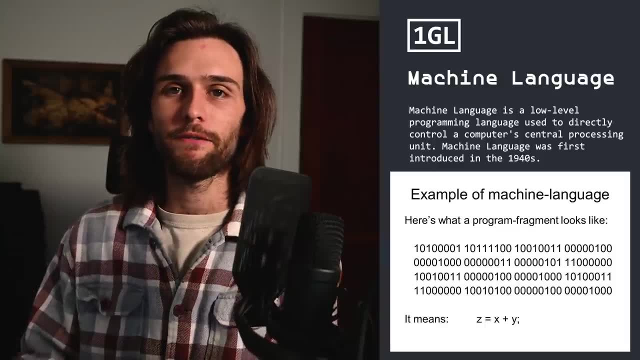 understand what I'm saying. it was very handy for the machine to understand. it was a lot more difficult for the human to understand. Now, while that is a disadvantage, it was also a perk, because this made for very fast and very efficient code. 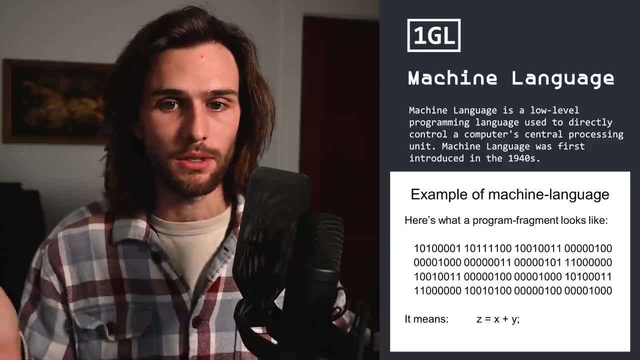 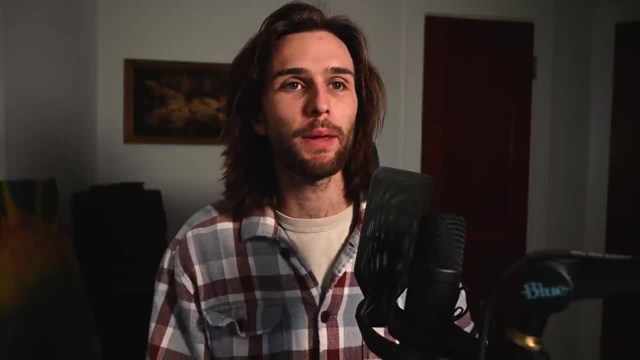 Because it didn't have to go through any assembler compiler. it converted, It was inputted directly into the CPU. And, before you say anything, yeah, well, supposedly yeah, that people still use this to code, or it's they statement called instructions you enter the instructions into. well, in this case it was called code. 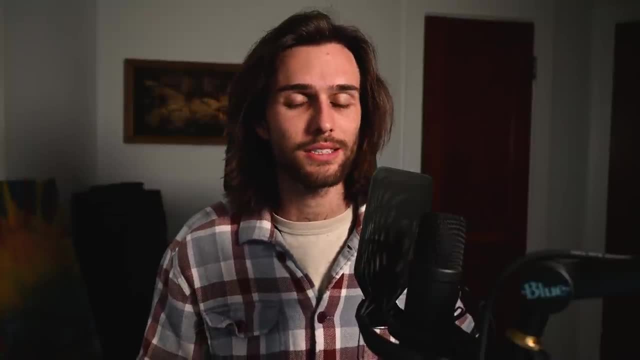 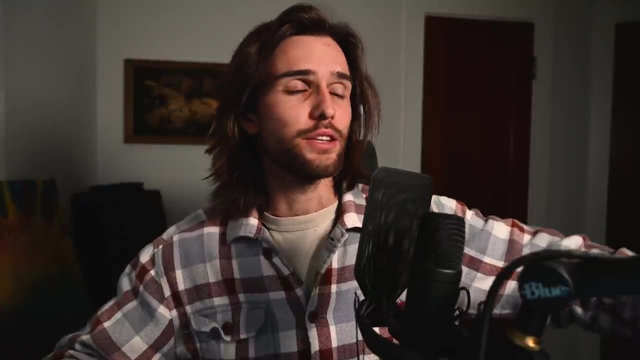 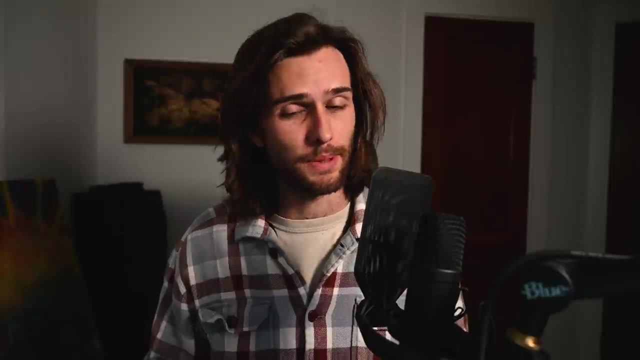 well, in this case directly into the cpu and it is executed by the cpu. but instructions code, yeah, but supposedly it's still used to program lower level functions of the computer, like, like, like the drivers or firmware hardware interfaces. it's kind of weird to hear that people still use this. 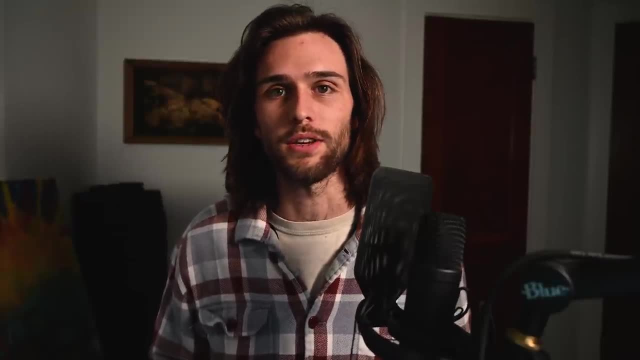 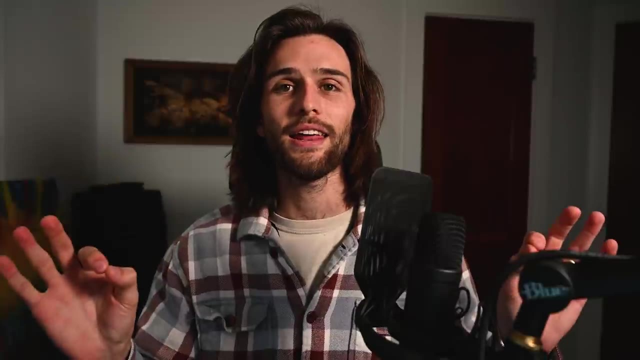 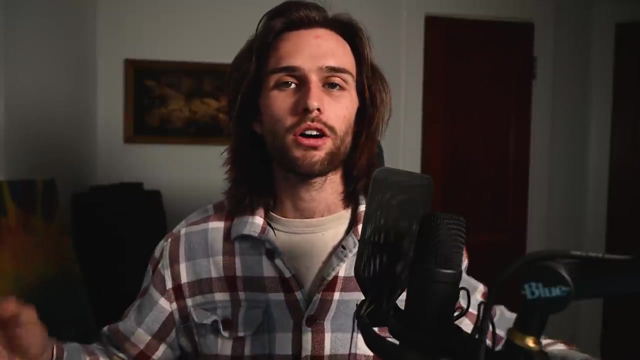 but that's what my research told me, so that's what i'm telling you. and just so you understand: 1gl, machine code, machine language, whatever you want to call it. that is well. basically, when you have your fancy 3gl plus languages like java and python, our compilers use that code to produce machine. 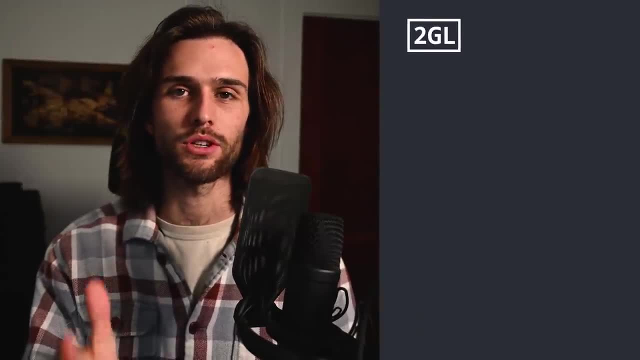 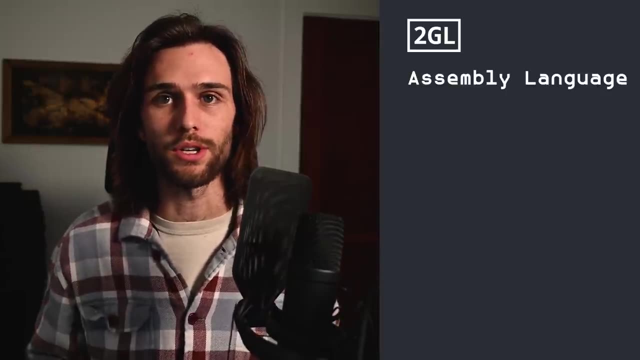 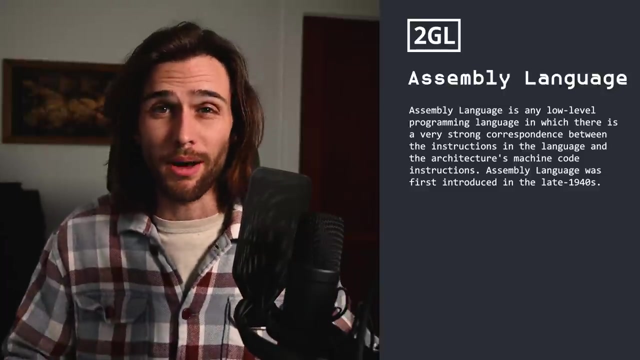 language for our computers to understand. the second generation programming languages are languages associated with assembly language. so we started with 1gl, machine language, now to 2gl, assembly language. this is our first ever look at a programming language that uses you alphabetical letters, english words, known as mnemonics- assembly mnemonics. that that's a huge. 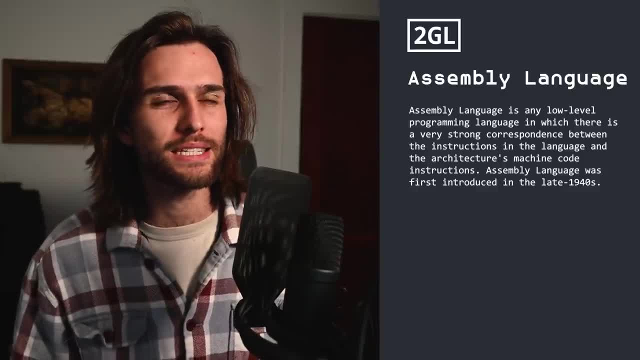 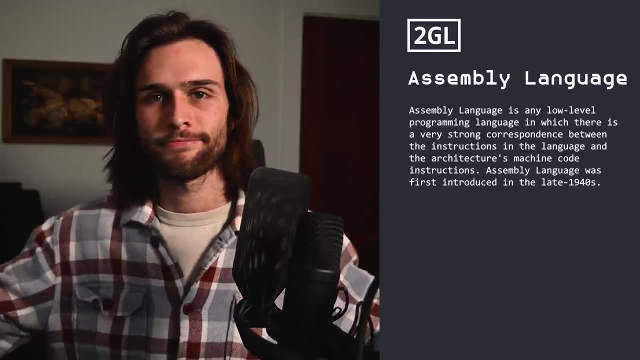 leap from just ones and zeros, and what's actually kind of funny about this is that you have some people arguing the fact that it originated in the 1940s and other people arguing the fact that it originated in the 1950s. i don't know why. this is a debate. let's set the record straight here. 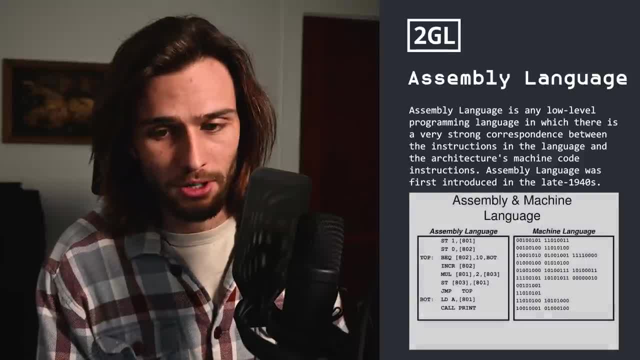 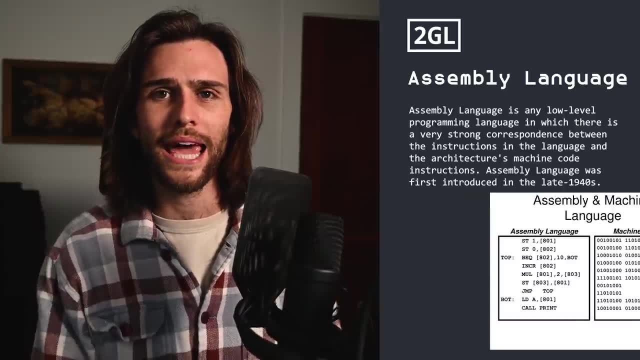 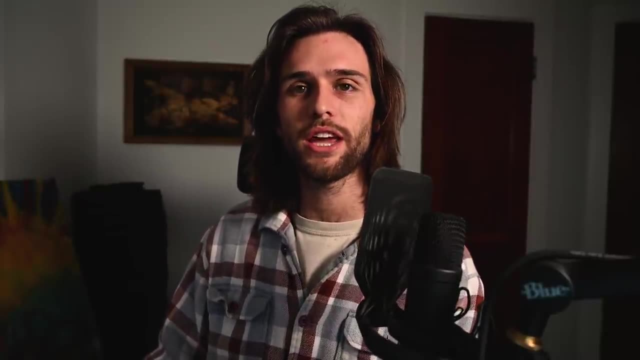 it originated in the 1940s. however, when you bring that up, it uh brings up another debate, and that is: was it? was it created by kathleen booth back in 1947 for the arc 2 system, or was it created by- uh, david j wheeler, that's his. 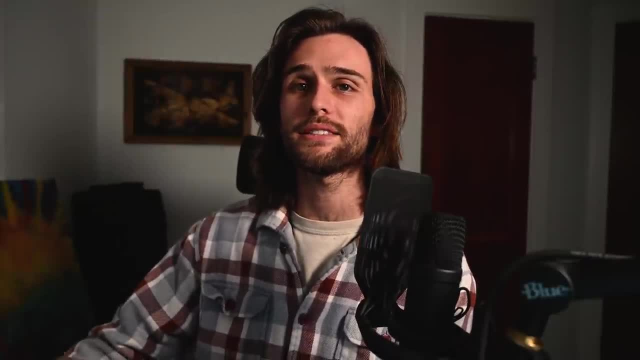 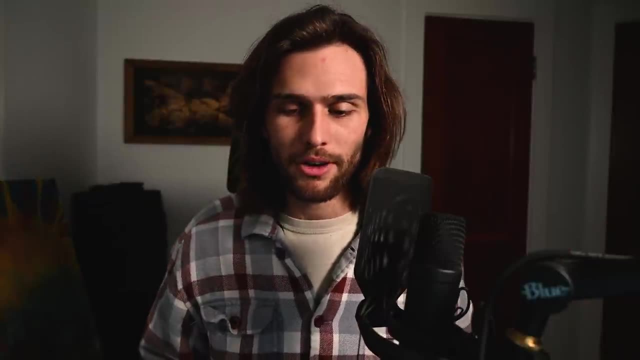 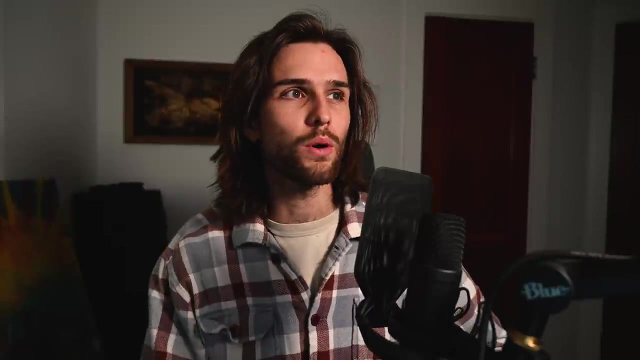 name right? yeah, david j wheeler for edsac in 1949. well, 1947 comes before 49, so i would have to say booth. however, i'm assuming the main argument comes from the fact that it appears that that kathleen booth's first assembly language was more, was more uh, based on mathematical operations where 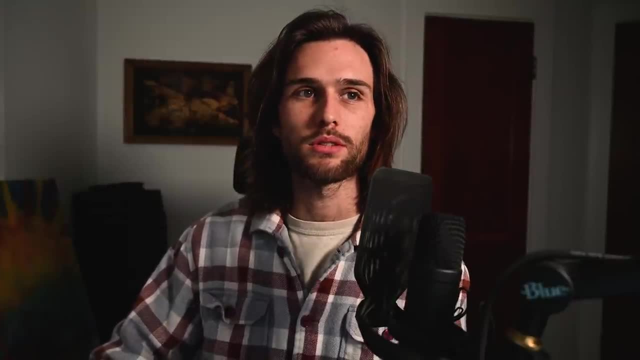 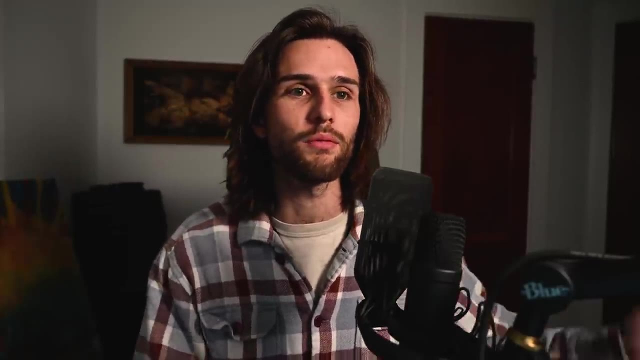 when it comes to wheeler's first assembly language- it was the first ever mnemonic based, so really heavily you know english words, alphabet letters, rather than what booth did in 1947. whatever it may be- and i understand people may be a bit more passionate about this topic- 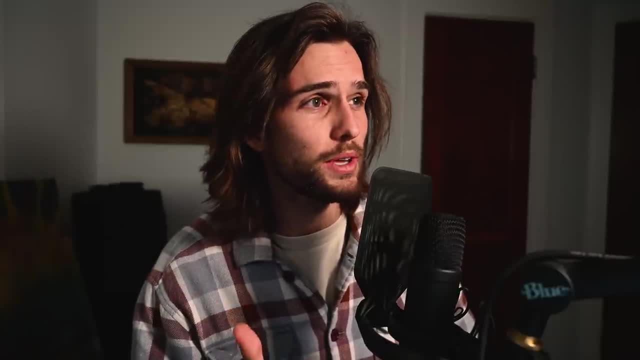 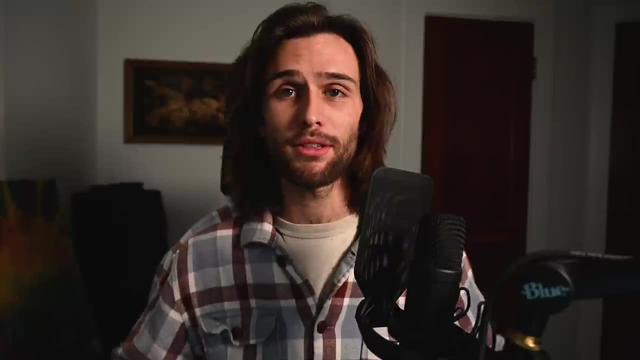 just for the record, women played a huge role in programming computer science around this time, and that's not me simping, that's just the truth. but either way, that can be a debate for another time. either way, it was originated in 1940s. i think the main argument for this is that it was a 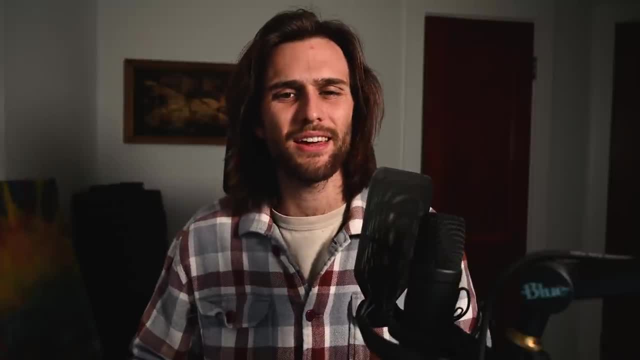 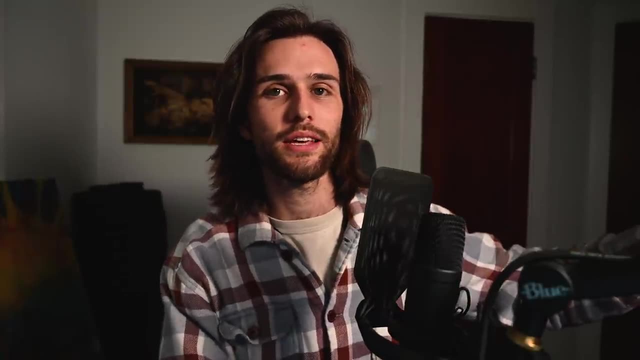 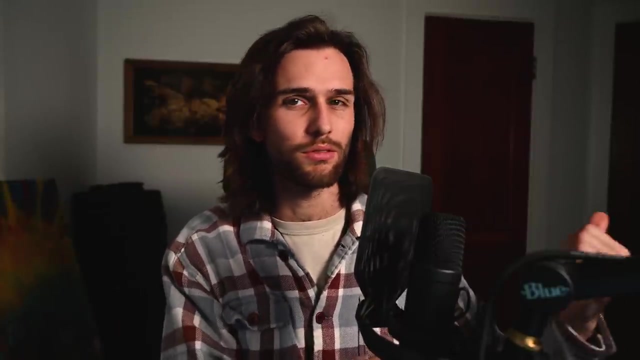 argument for why it- some people say it was uh- originated in the 1950s. well, i have three theories. one was: maybe it's just because of how much it progressed in the 1950s and it got more of a, a solid- this is assembly language- feel in the 1950s, even though it's still originally in 1940s. or 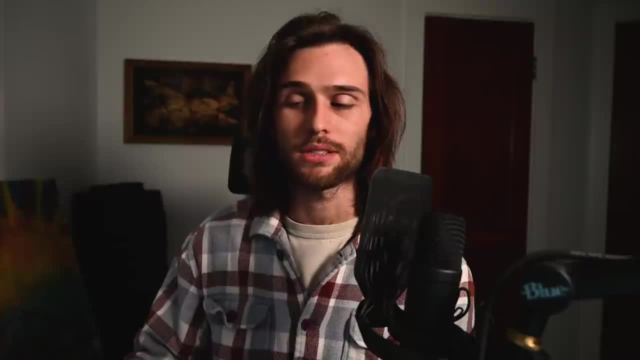 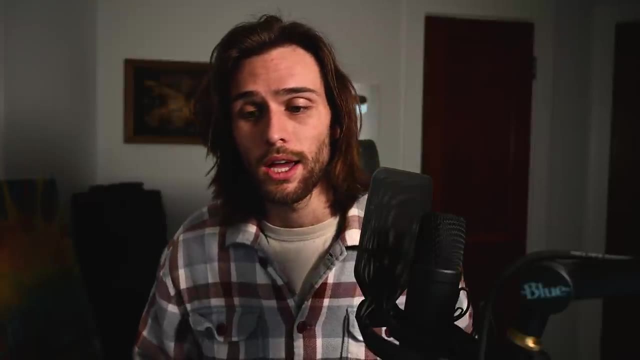 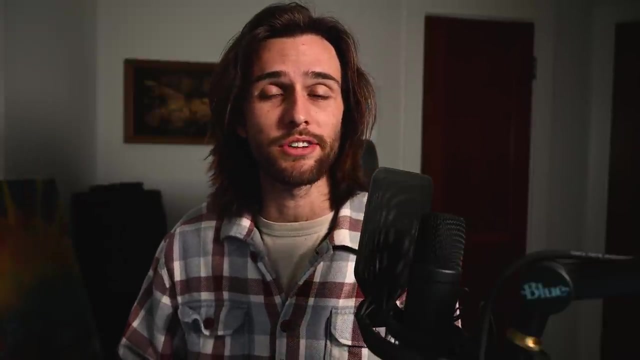 it's because it wasn't popular until the, the 1950s, or the late 1950s actually, or- and in all honesty this one is just as likely as the previous two- someone accidentally mistyped 1950s instead of 1940s, so now you have all these lackluster researchers regurgitating 1950s without 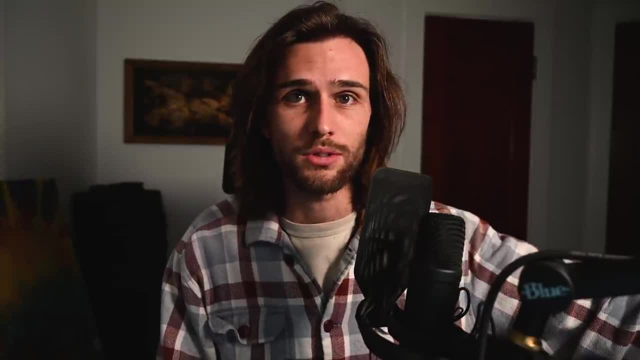 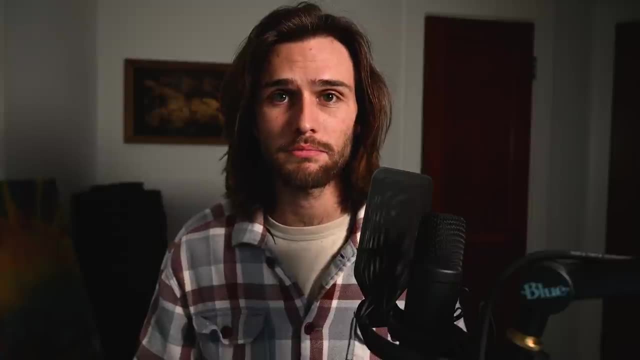 actually doing any research other than whoever made the initial typo in the first place, and it just kind of spread throughout the internet from there. back to the actual language. now we're still not using a compiler, but this is assembly language, so we are using a, an assembler, to convert this. 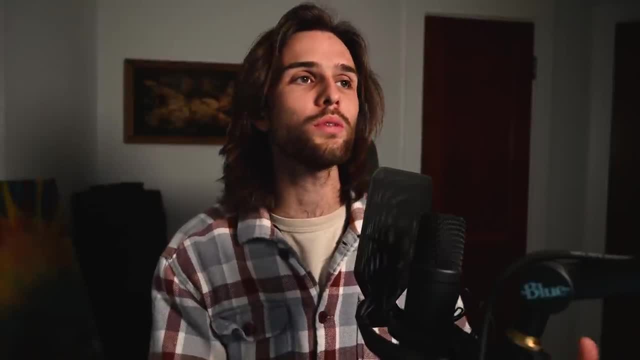 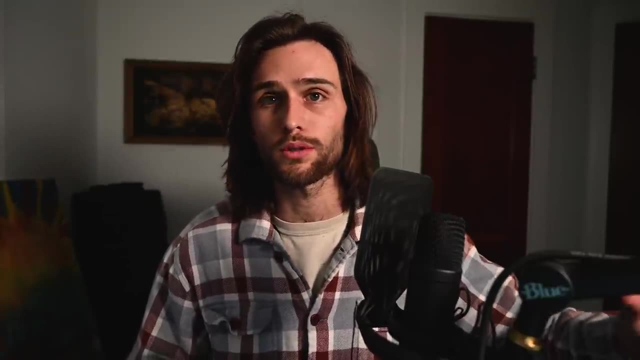 language into a compiler, into machine language, and this was huge. not only did assembly language allow for easier human readability, but the assembler made it a lot easier for actual debugging and also introduced more advanced methods of programming like macro and structural programming. and while it is a big step, 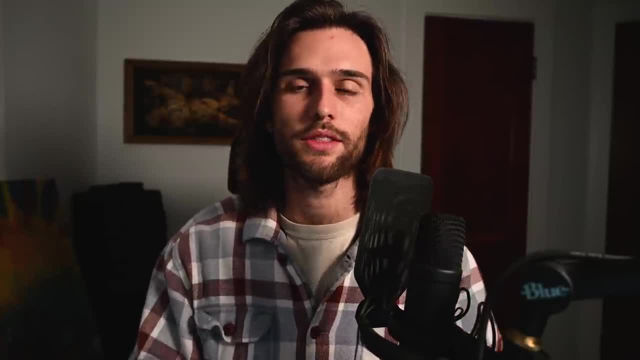 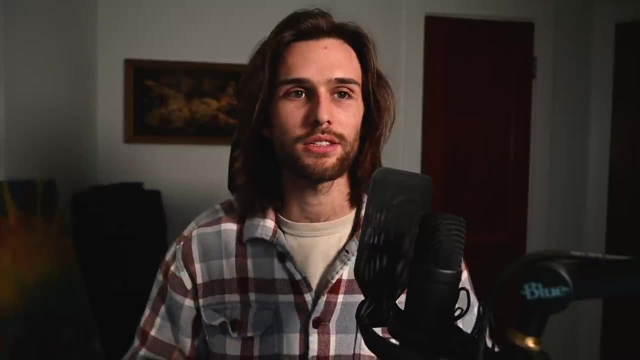 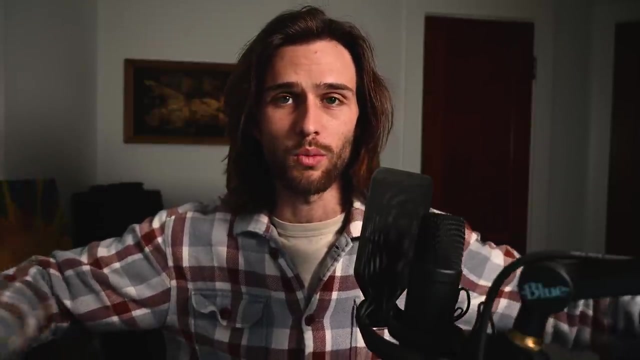 for machine language- remember this is still a low level language. they're mostly used in low level kernels and drivers and for like process oriented, performance based applications like video editing or computer games or graphic manipulation applications. and that's it for the low level languages. 1gl- machine language. 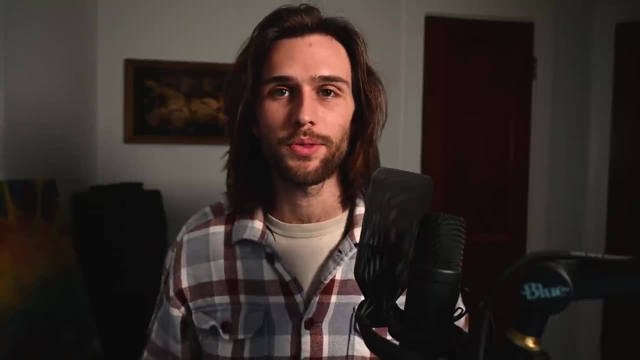 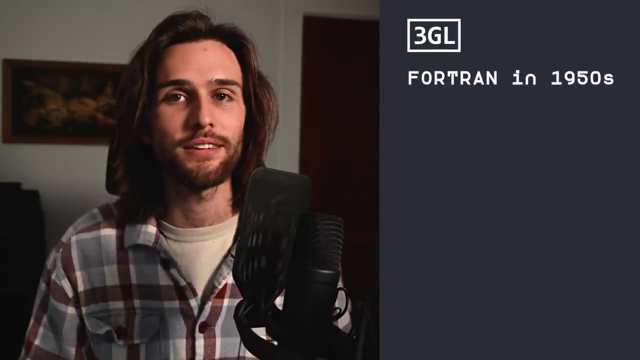 2gl assembly language. now 3gl, the third generation programming languages, is our first look at a high level language, the first few being fortran in the 1950s, basic in the 1960s, pascal and c in the 1970s. 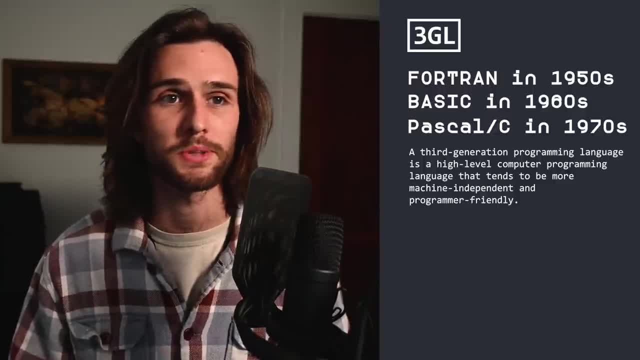 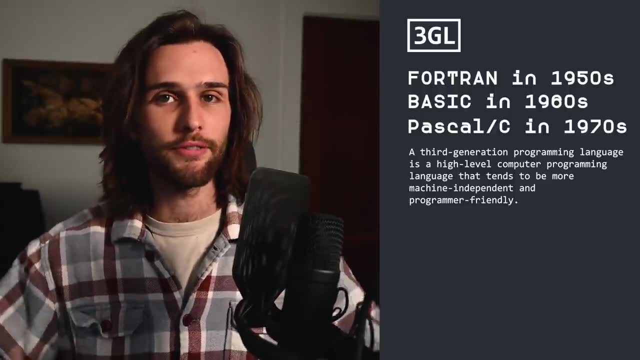 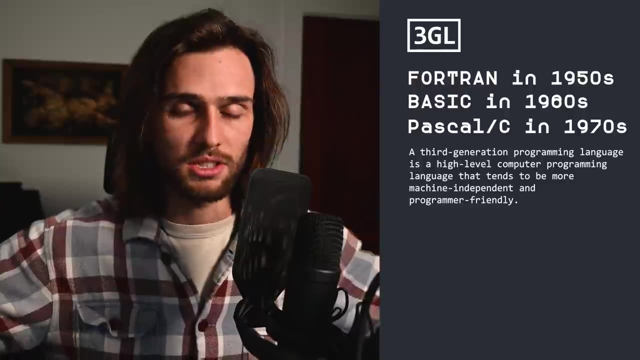 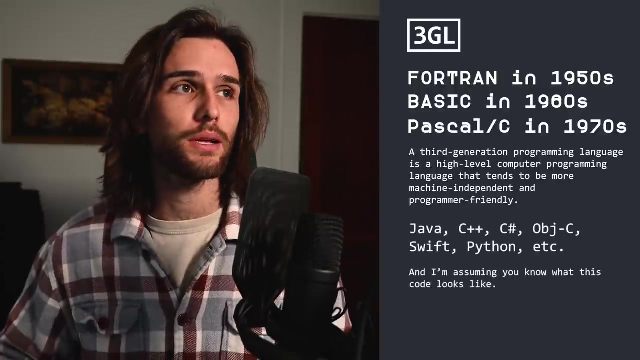 and so on. this was our first introduction into variables, constants, loops, error handling, aggregate data types, flow constructs. but the main reason we're using a high level language is because we're emaing to be able to convert a machine language to c. it's the magic we want, but one of the other reasons why we don't have 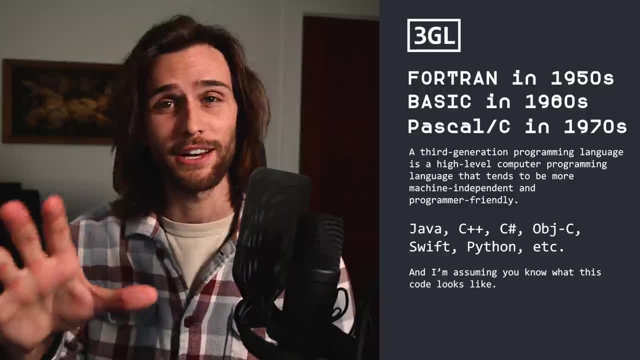 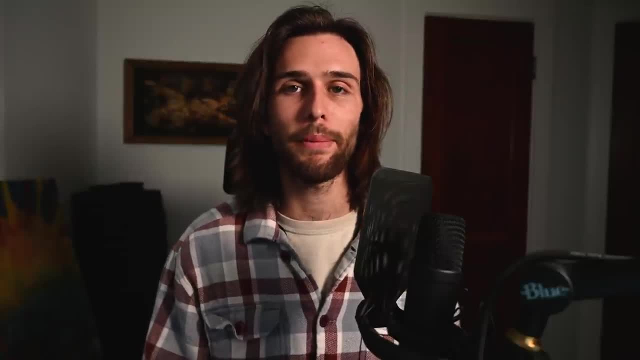 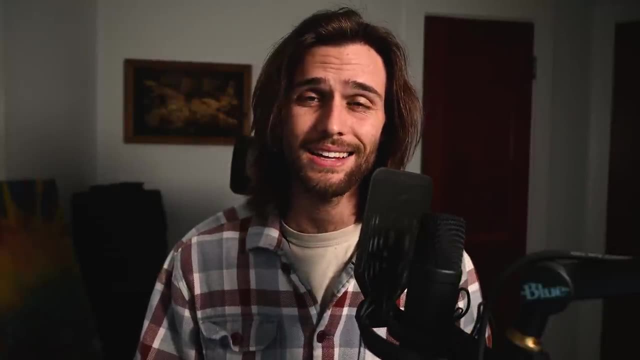 to utilise knight is because we know that key language programming supports this mathematical transition process, and that's why we're using these programming languages, whether they're animated or visible. we don't need to have a compiler to convert our code as a technical or object code, which, by the way, a compiler was first introduced back in 1952.. This part is: 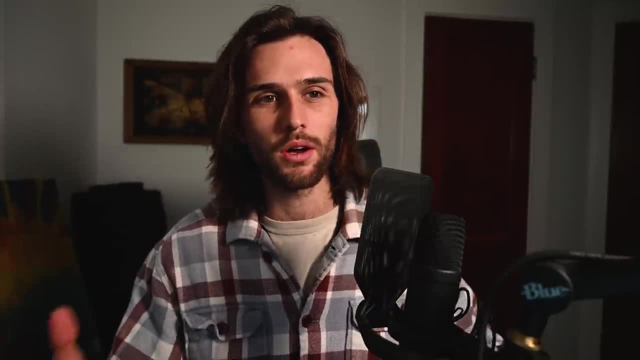 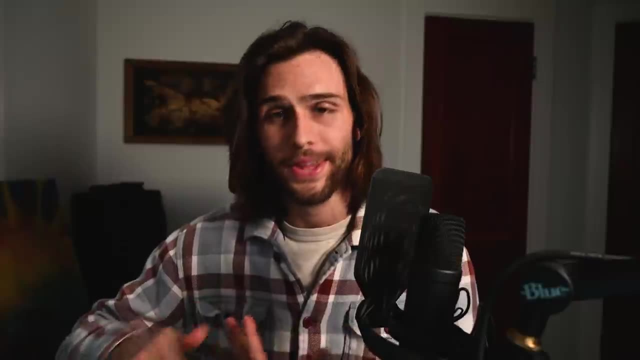 typically when I say the uses for these languages, but I feel like we all know. you know how you use Java and C++ and C sharp. And as much as I want to hop right into 4GL, I can't just yet because 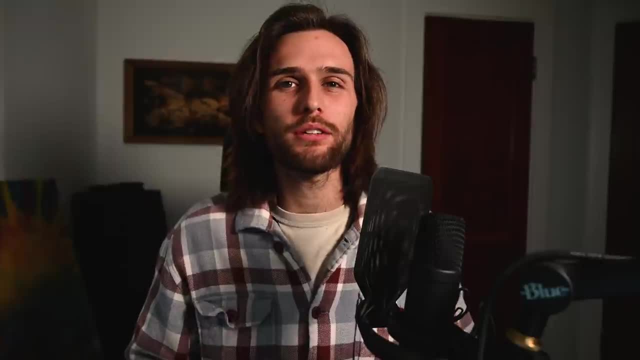 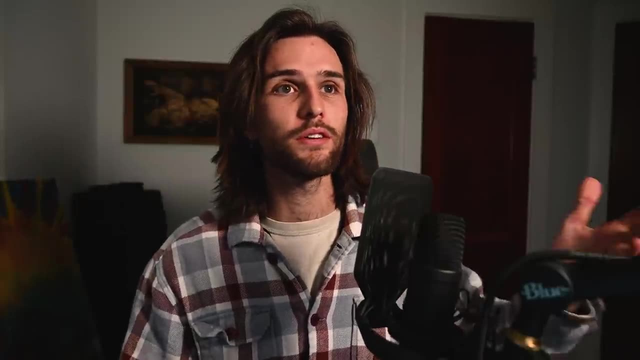 there is another debate. I don't know why people just can't agree on these things. That is, Python, Ruby, JavaScript and a couple others lumped in there. Some people consider these 4GL, while other people consider these advanced 3GL Based on everything I see. I also consider these. 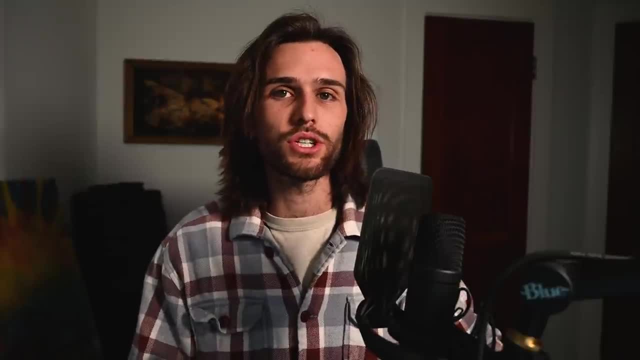 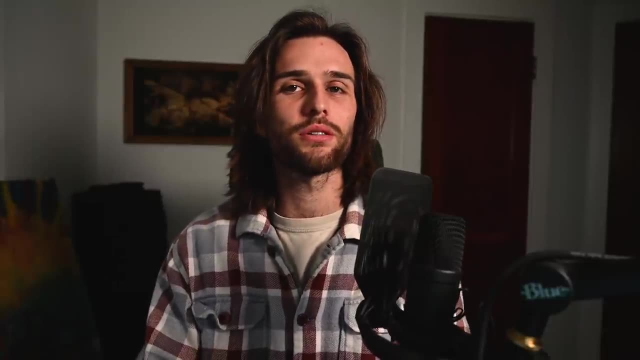 3GL. The thing is, it's it. these 3GL languages have 4GL abilities and features, but just in a 3GL environment And, to be honest with you, I think that's the general consensus that these 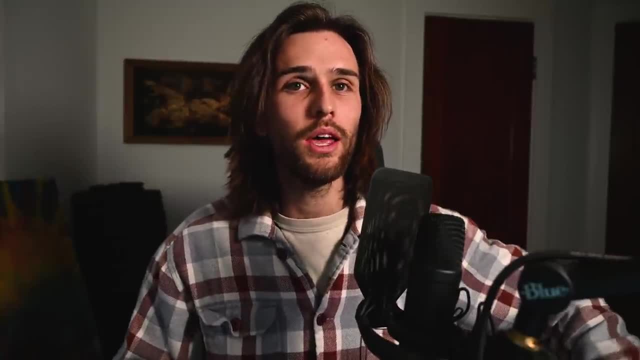 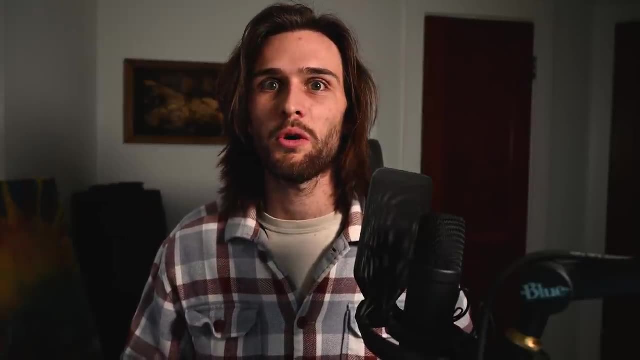 are all 3GL languages, with the exception of just a few. Maybe those few are just really loud, In all honesty, maybe- and this is just like a theory- a code theory- No, this is just a theory, I think. 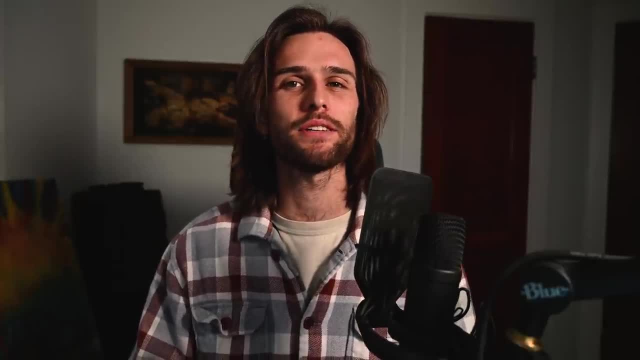 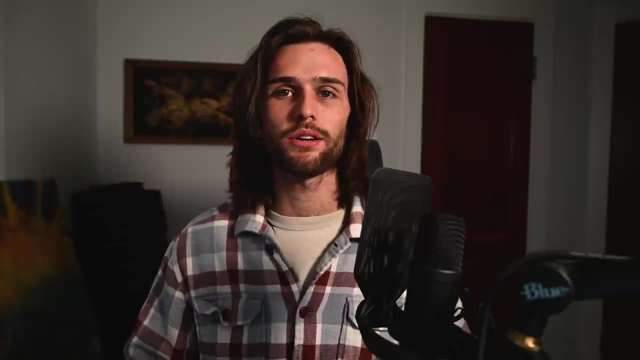 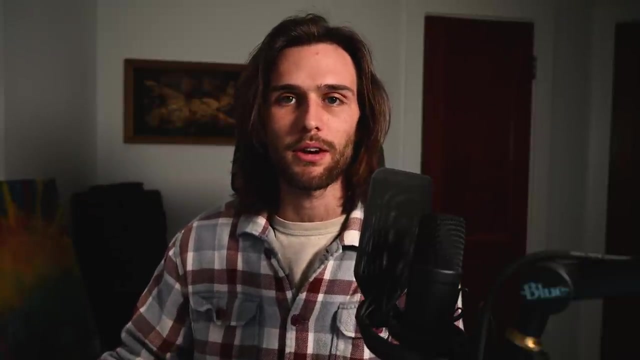 I think that people may have considered these 4GL when they first came out, but retrospectively looking at it, now that we know what is considered 3GL and what is considered 4GL, they definitely fit in the category of 3GL, much better than a 4GL language which we're about to talk. 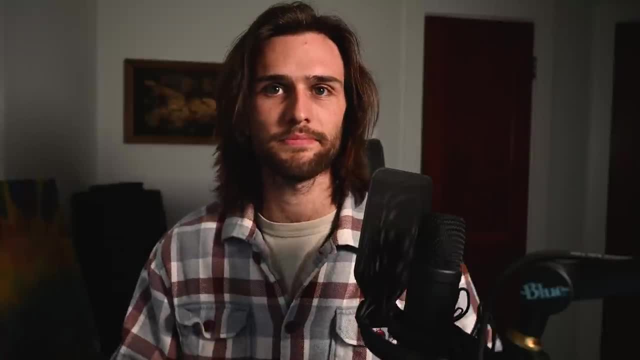 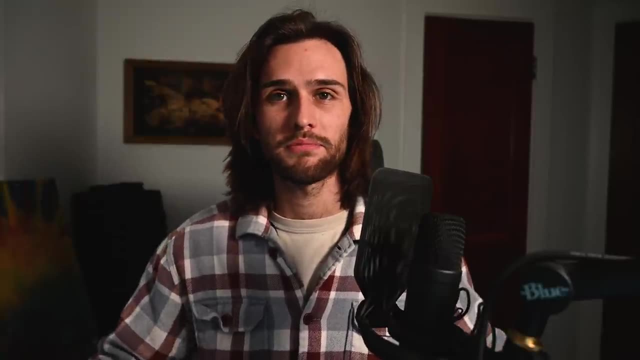 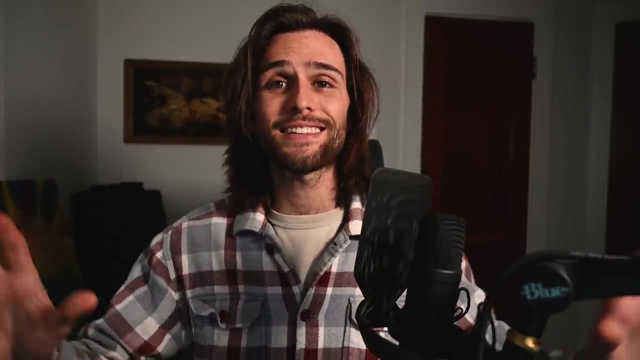 about in a second, Not to mention the fact that definitions for these particular things change over time and how it's changed over time. all of it just leads to me saying that Python, Ruby, JavaScript are 3GL languages. I just felt like I needed to say that. 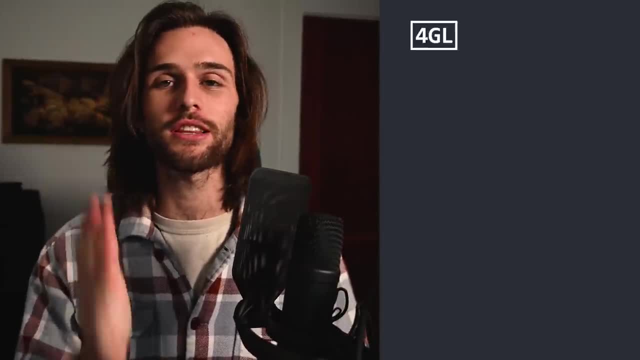 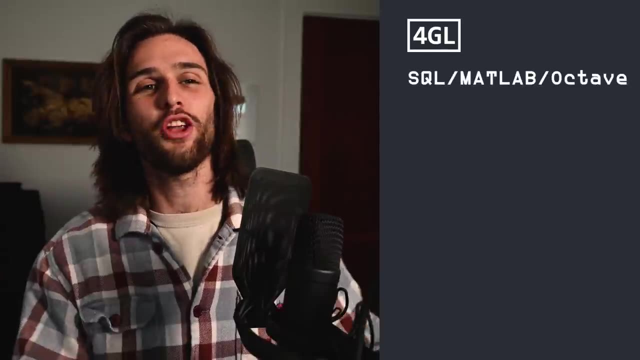 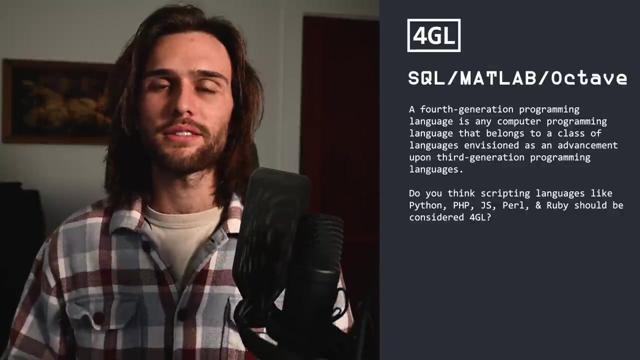 Now the real. the real, the fourth generation languages are just another step closer into having a more human, another step closer to human language form of thinking, conceptualization, That's the best way for me to put it- And considering the previous sentiment of not knowing which exact languages are 4GL. 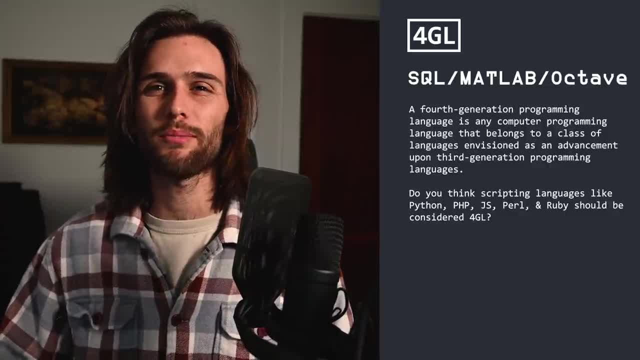 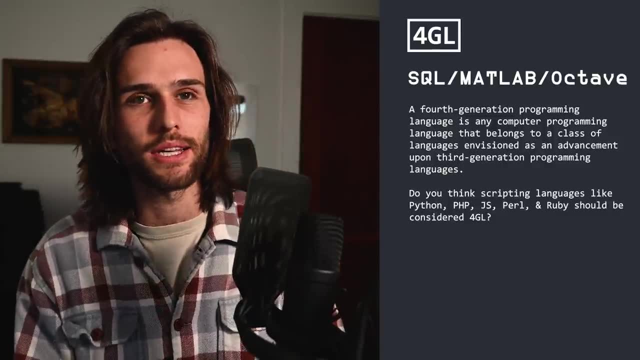 or what may or may not have been the first 4GL language. it's hard for me to put a date on when exactly it originated. However, SQL originated in the 1970s. SQL is a 4GL, a fourth generation language, with many current 4GL languages being based. 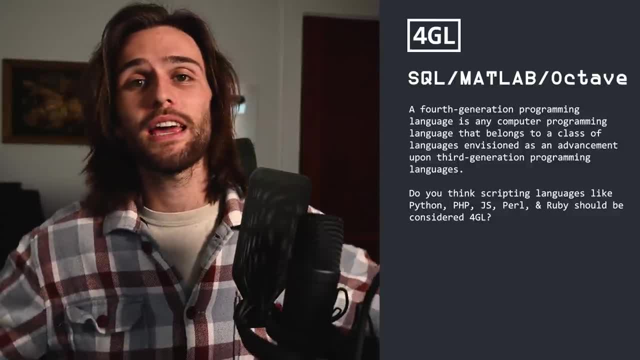 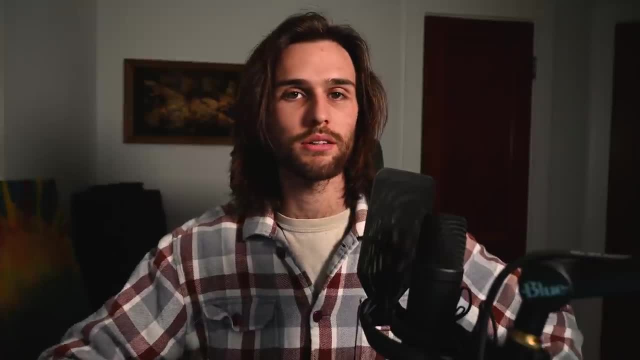 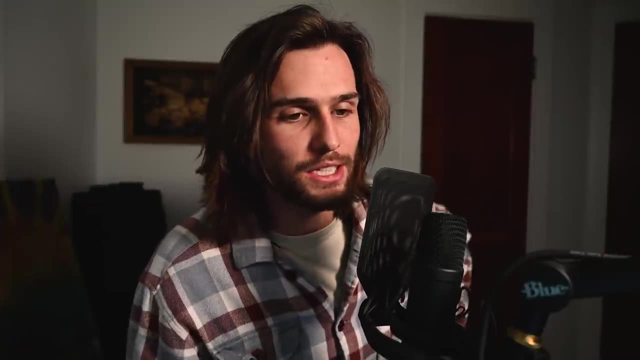 on SQL, SQL, whatever. So I'm going to have to say the 1970s. The main domains for 4GL are typically dashed Database related, like database queries and reporting and things that have to do with the database. Let me read off most of the domains for it. 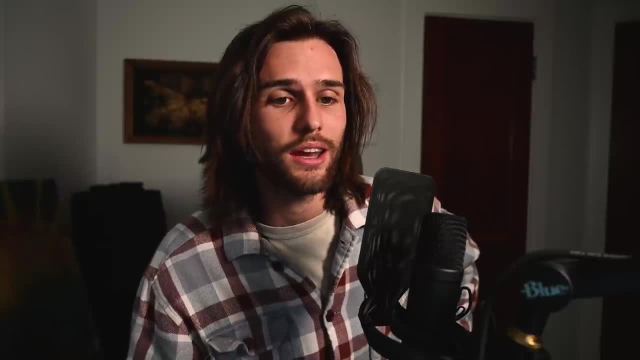 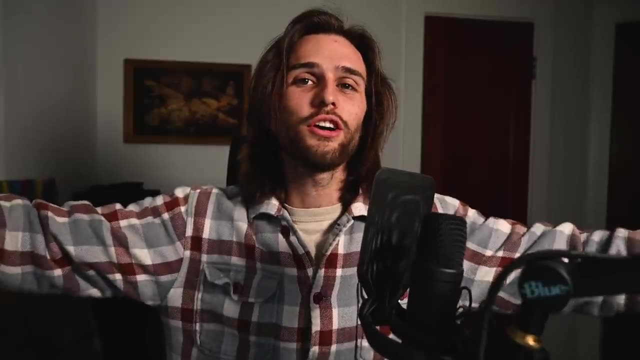 You have database queries, report generators, data manipulation, analysis and reporting, GUI creators, screen painters and generators and some web development languages, And there are actually a good amount of 4GL languages, but some you may recognize, of course, are SQL. 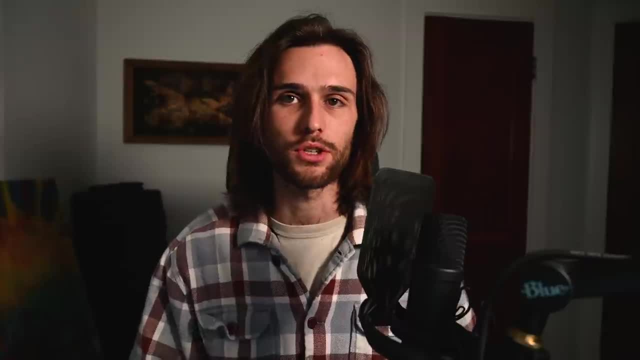 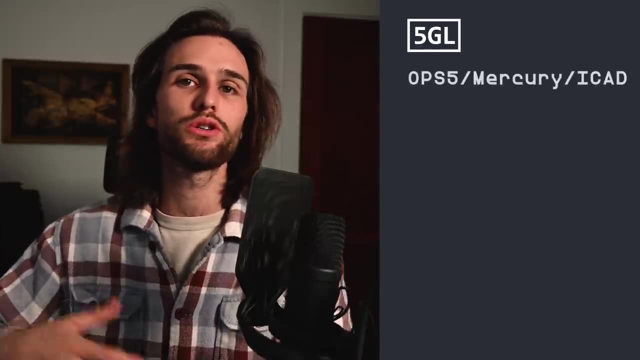 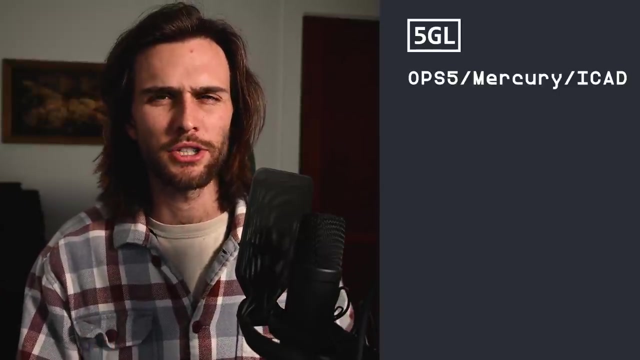 There's also Octave, MATLAB and Progress 4GL. The fifth generation programming languages are 4GL. These programming languages are really focused on constraint-based languages and some use visual tools to help you develop. But when I say constraint-based languages, that's basically replacing our job. 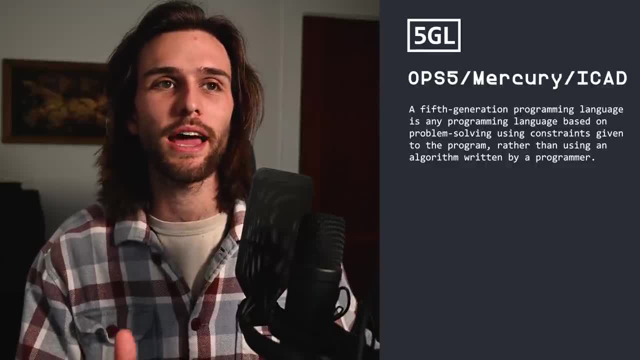 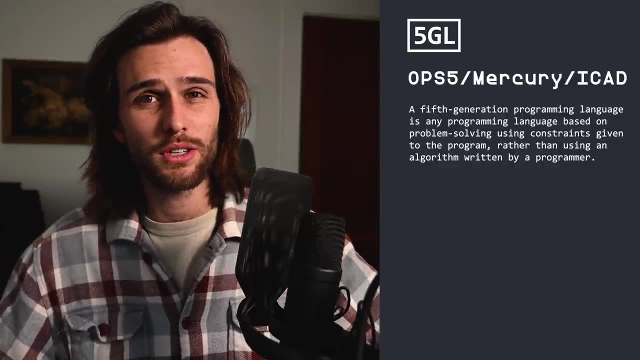 We created to replace our job. Constraint-based languages are languages that basically solve the problem without the use of the programmer, Kind of like artificial intelligence in there. a few other domains in there: OPS 5, KL1.. I know there's a couple more. 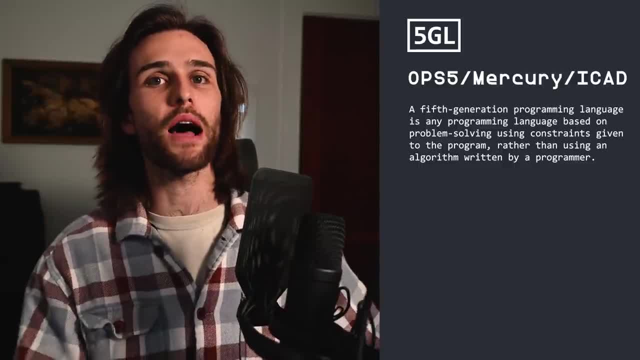 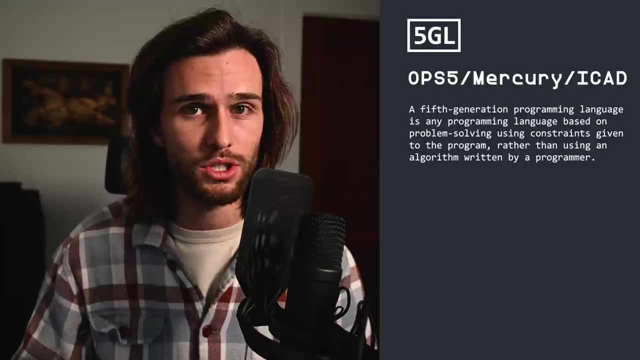 Mercury and ICAD. Those are all examples of 5GL languages. And I know I'm being redundant when I say 5GL languages, because that's me saying fifth generation language languages, But it rolls off the tongue better. And if you haven't heard of these languages, not a problem, because I haven't either. 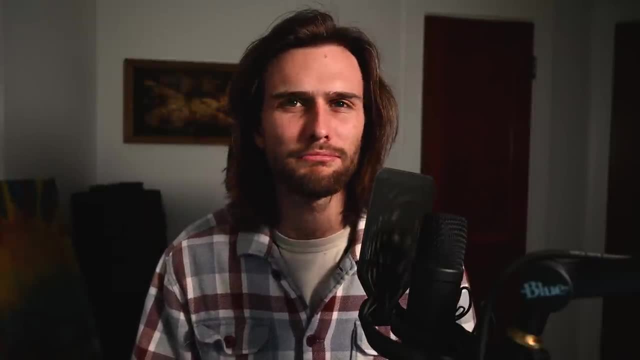 I feel like I've heard of ICAB, but I think I'm just confusing it with AutoCAD. Probably The thing is, in the 1980s, 5GLs were thought of the way of the future. That all. 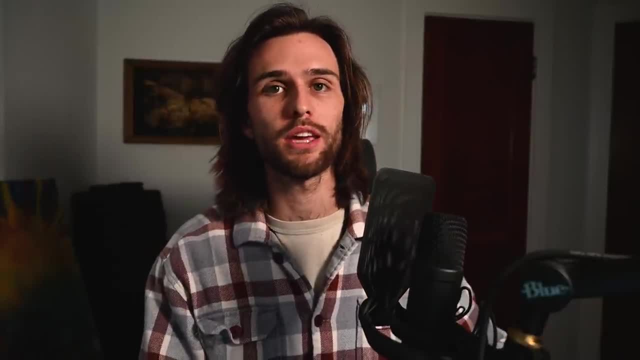 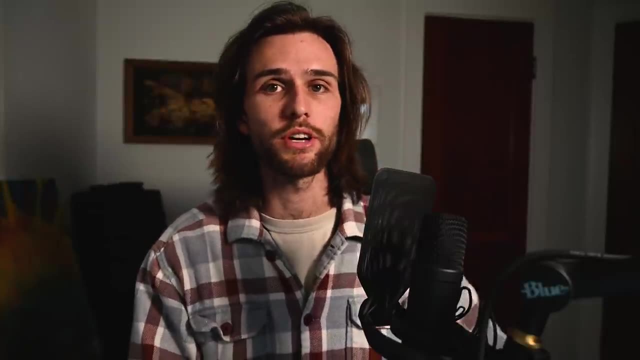 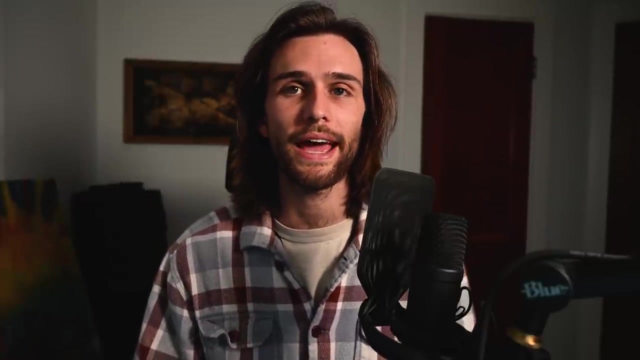 procedural programming was going to be replaced with constraint-based programming. for one reason or another, Because of this, there was a bunch of money dumped into 5GL research and development back in the 1980s and 90s, But it proved to be a little more difficult than what they had thought, so it just kind. 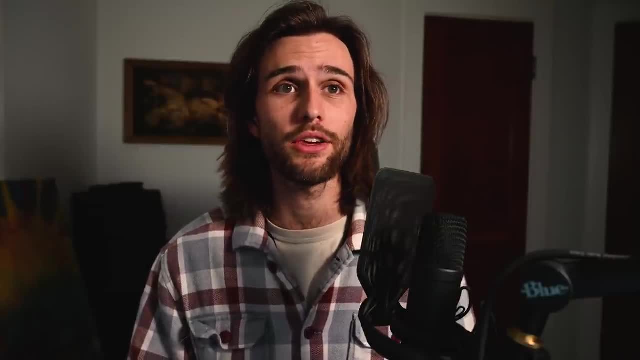 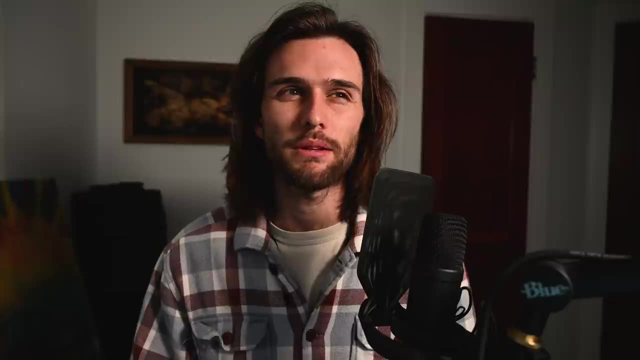 of fell off. I mean, I do remember back in college I used Prolog, which is supposedly a 5GL, a fifth-generation language, but that's the only time I've ever used Prolog. That's the only use case I could ever see myself for using Prolog. 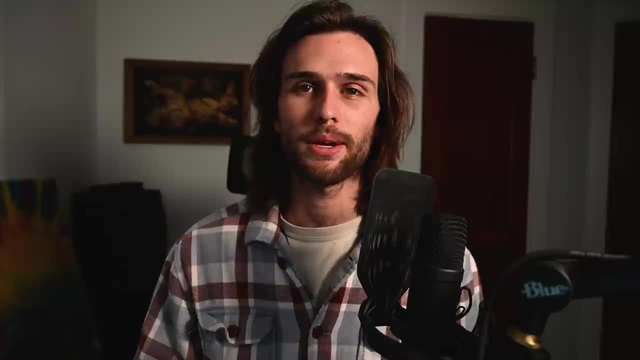 And that's basically where my knowledge of it ends And that's all I want to talk about on the topic. To be honest with you, it doesn't Who really cares if something is considered a 5GL or a 4GL or a 3GL. 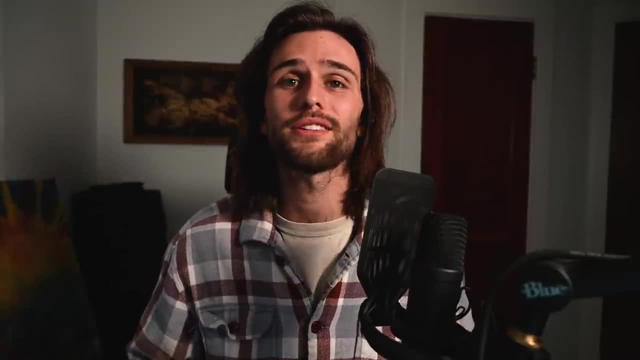 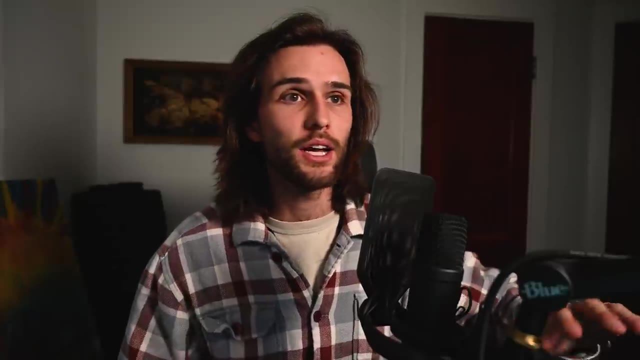 Like I don't know why people are arguing about whether or not Python is a 3GL or a 4GL. It doesn't really matter. I just wanted to make this video to talk about the history of programming languages and how it progressed from back in the 1980s. 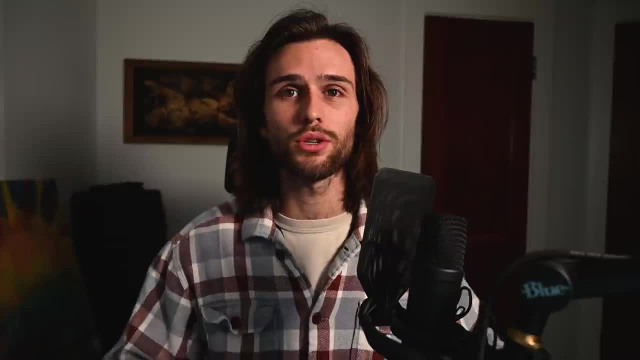 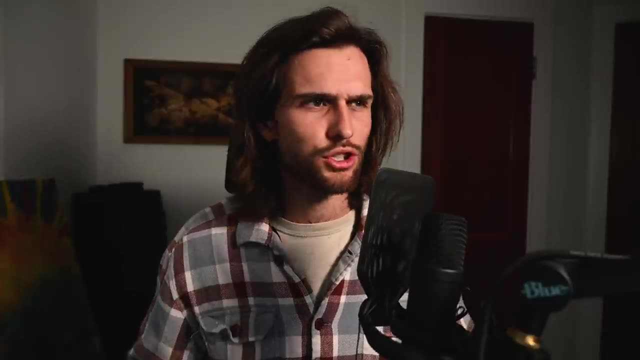 1940s, from machine language to assembly language to, you know, our beloved 3GLs, Java, Python, C++- I'm sure Swift would be considered in there as well- And then to 4GL and 5GL. that 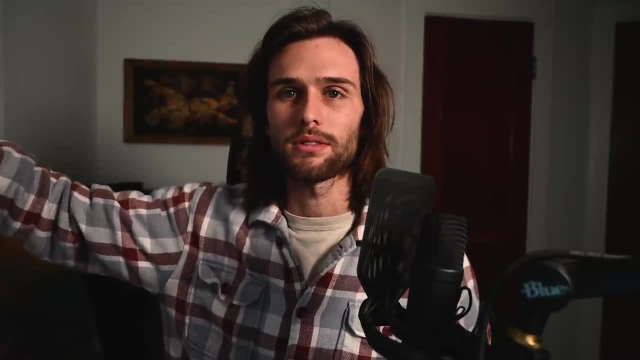 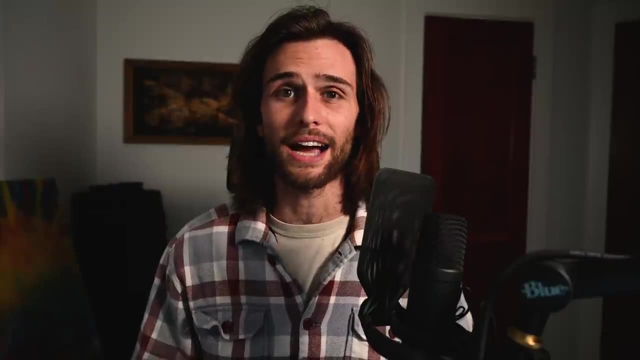 Well, 4GLs are actually very widely used, you know, with MATLAB and Octave and SQL of course. But then to 5GL, which if you ever use, If you use a 5GL like actually not just for a hobby, well even for a hobby, let me know. 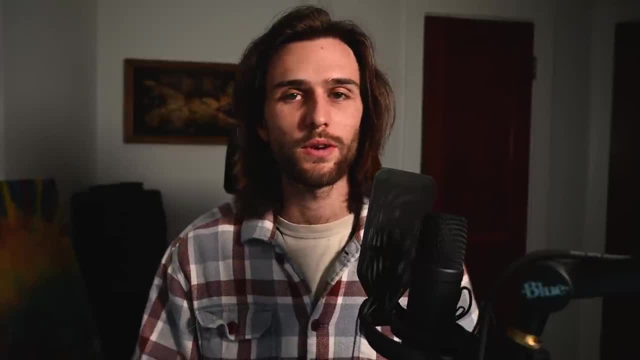 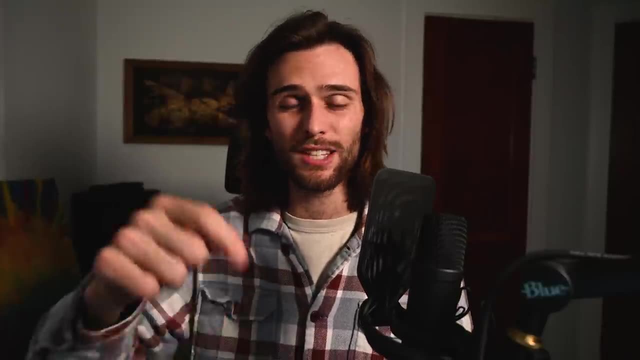 in the comment section. I'm genuinely curious. I would love to know- I hope you enjoyed watching this video as much as I did researching and making it- If you have any friends that you think would be interested in this type of content in. 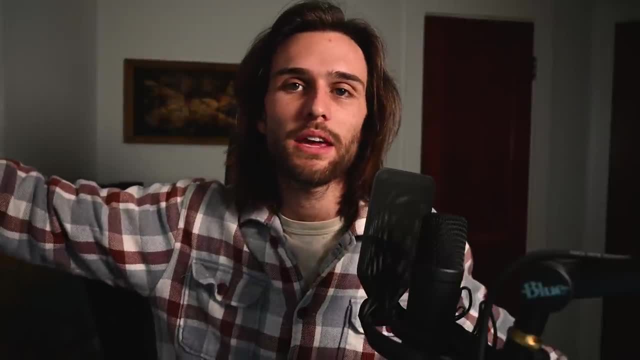 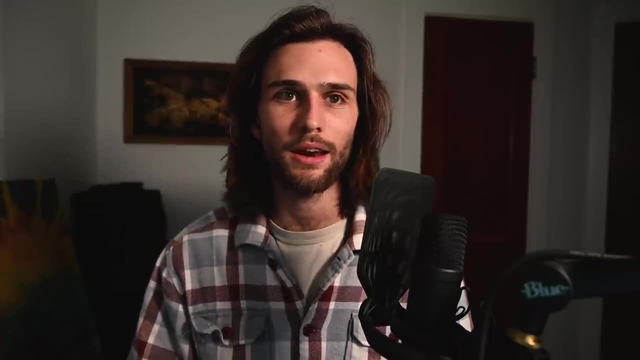 this video in particular. send it over to them and now you don't have to give them a Christmas present. It's a win-win. I would really appreciate a like on this video for algorithmic purposes And my analytics say that most actually a good amount, like 75% of all my viewers are. 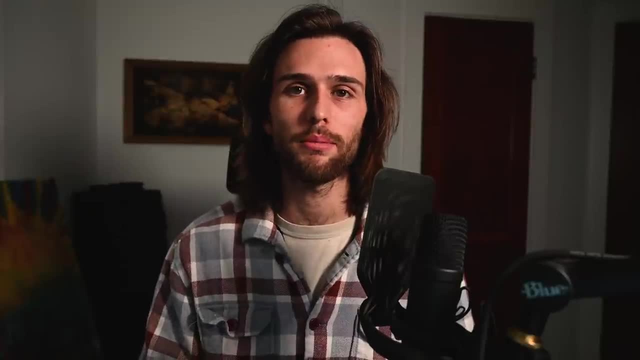 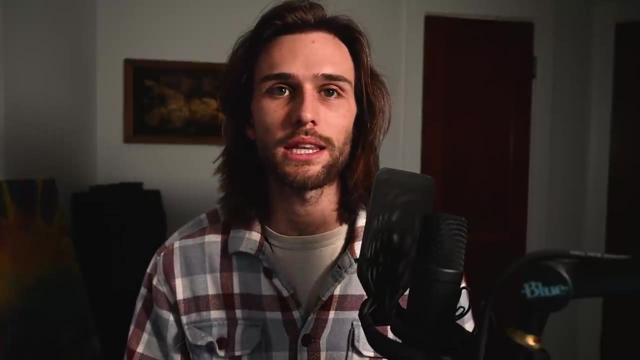 not subscribed, So make sure you're subscribed. Look at the subscribe button, Especially if you made it this far In this video. that means you at least a little bit like the content I have to make, and I make a lot of videos like this.